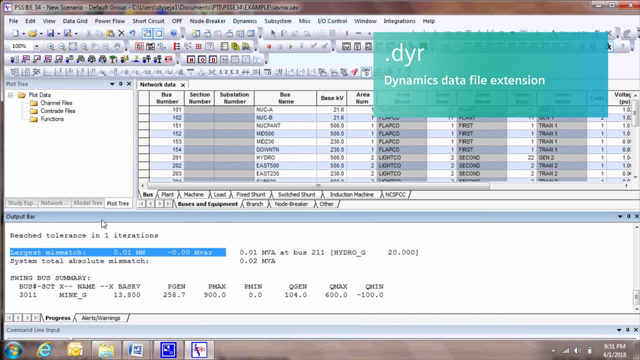 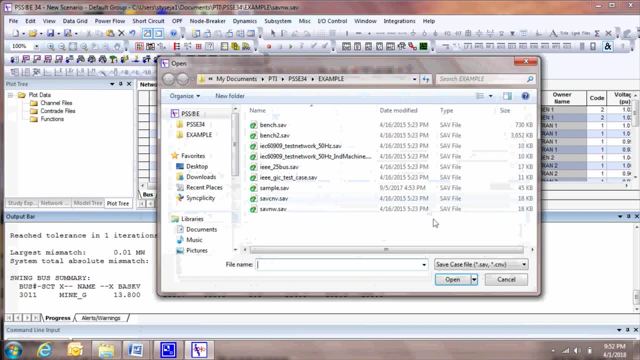 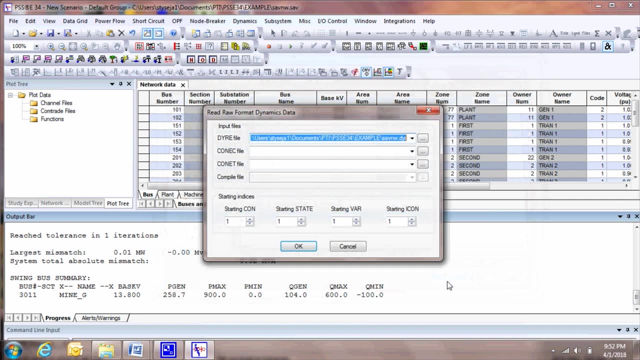 will use for this illustration is the SAVNWDYR. To read the dynamics data, go to File Open and select the file type: Dynamics Data File. select the file SAVNWDYR and select Open. This opens a dialog where you will see the. 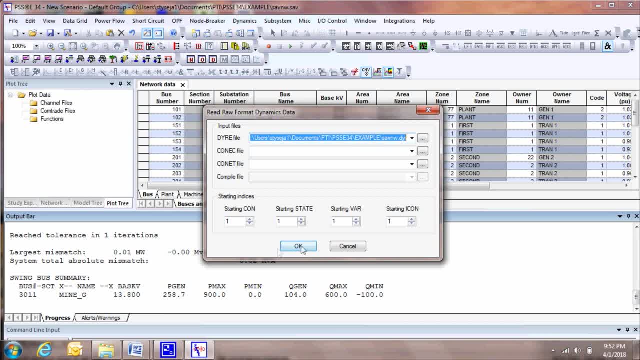 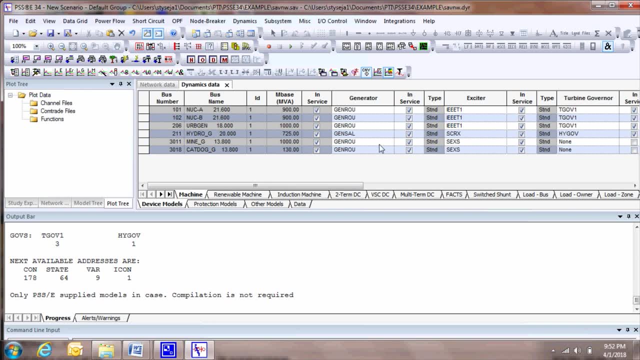 name of the DYR file you just selected. Click OK and PSSE reads in the dynamics data. You can now conduct the dynamic simulation. Before you do this, you may want to define the plot variables to be viewed after carrying out a dynamic simulation- One quick and easy. 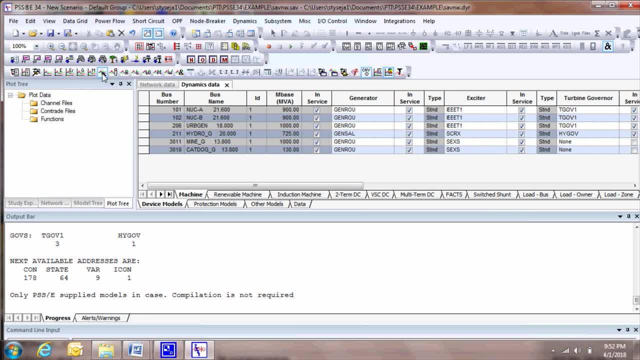 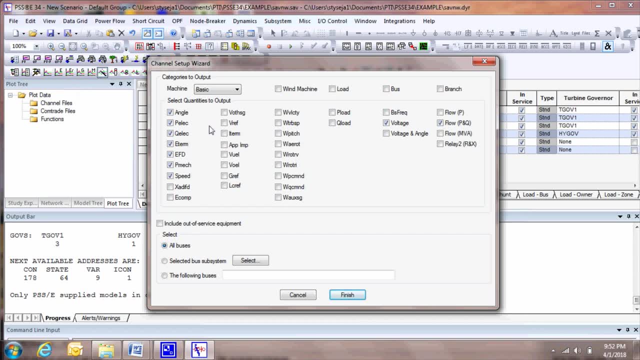 way to add the plot quantities is to open the Channel Setup window. To do this, you can go to the Channel Setup wizard and select the quantities you wish to plot. For the purpose of this example, we'll select All Buses and click Finish. All plot quantities are added. 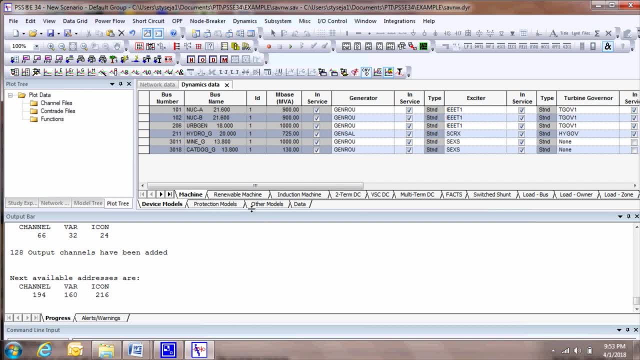 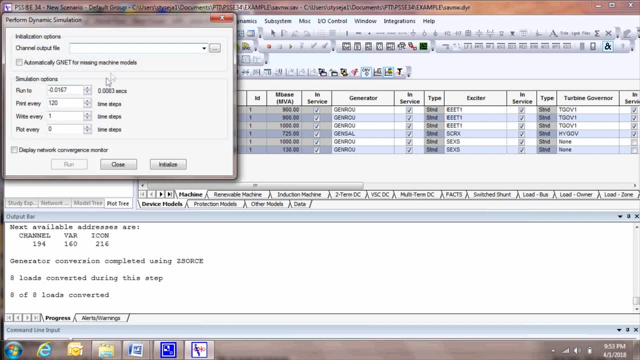 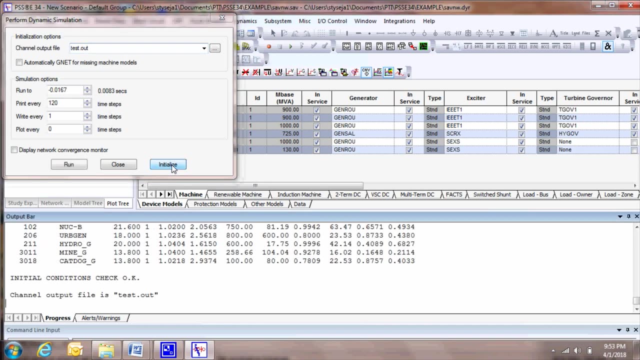 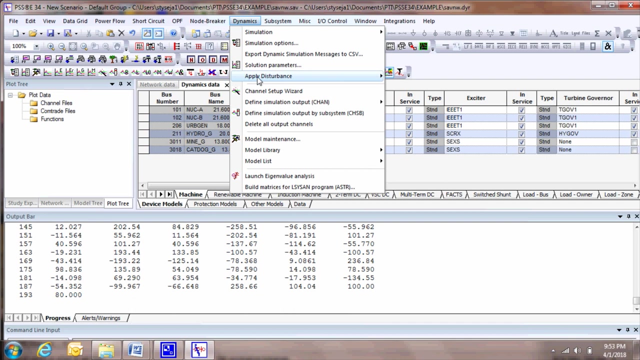 to the dynamic case. To run a dynamic simulation, select the Dynamic Simulation Toolbar icon and specify the name of the plot output file. Then select Initialize. Before you apply any disturbance, you should run the simulation flat for a few seconds To apply disturbance. go to Dynamics: Apply Disturbance. We will apply a 6-cycle 3-phase. 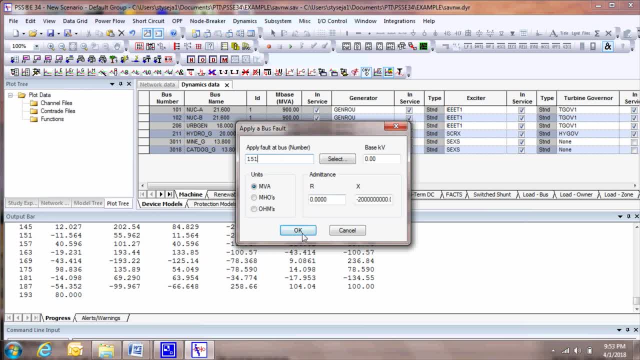 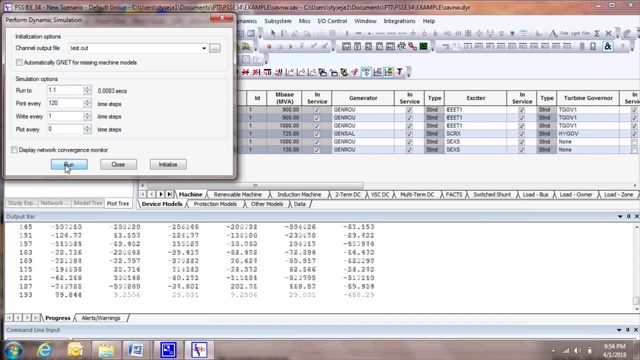 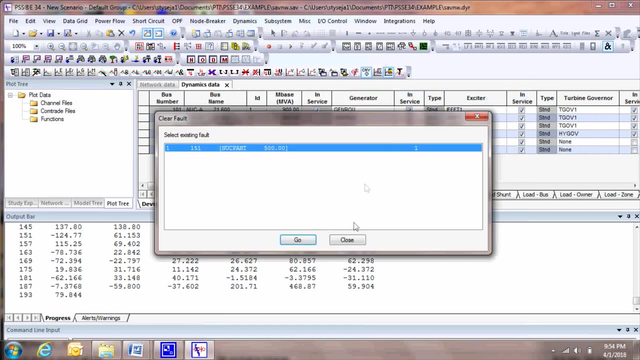 bus fault at bus 151. Run with the fault for 6 cycles and then clear it. Choose Dynamics, Apply Disturbance and click Finish. All plot quantities are added to the dynamic simulation. To run the dynamic simulation again for 10 seconds To get a better understanding of: 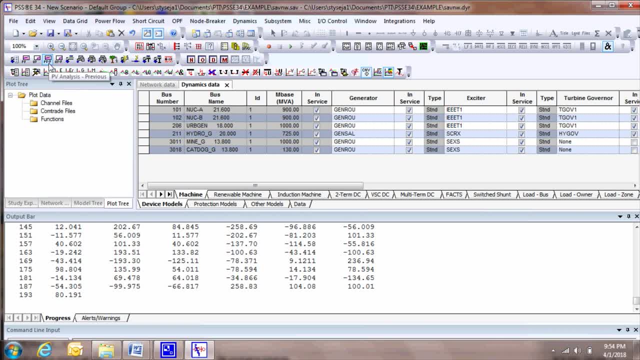 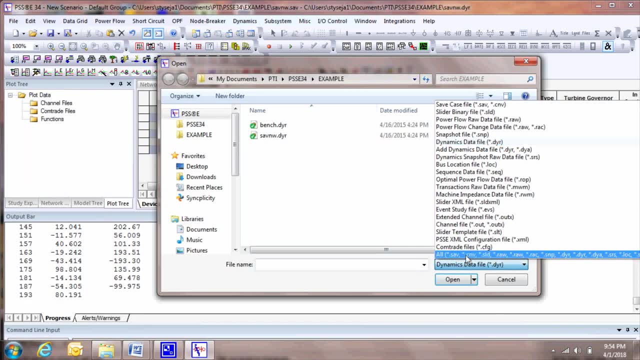 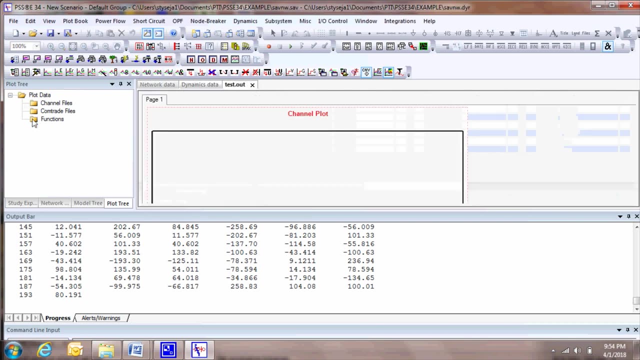 the dynamic simulation results. you can review the Output Plot Quantities. Click File Open and open the test you just generated. You'll see the file with all the plot quantities and all the channels on the tree view. You can drag and drop the plot to better understand. 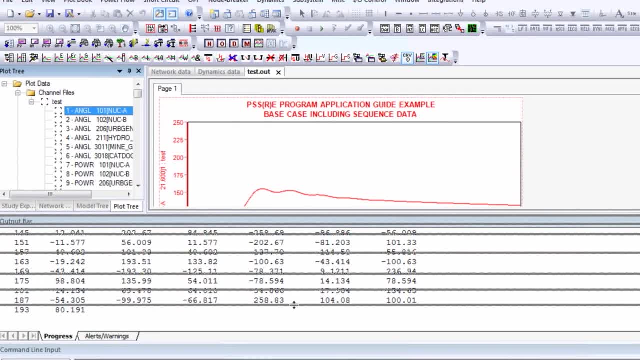 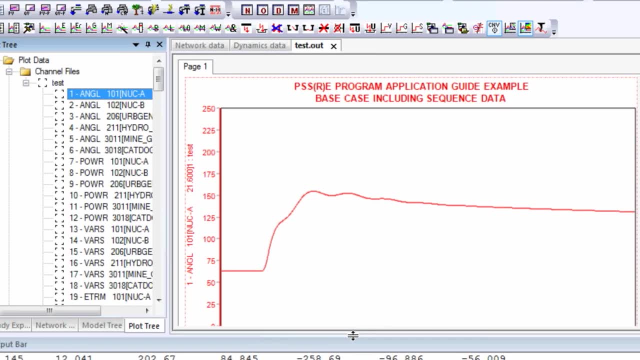 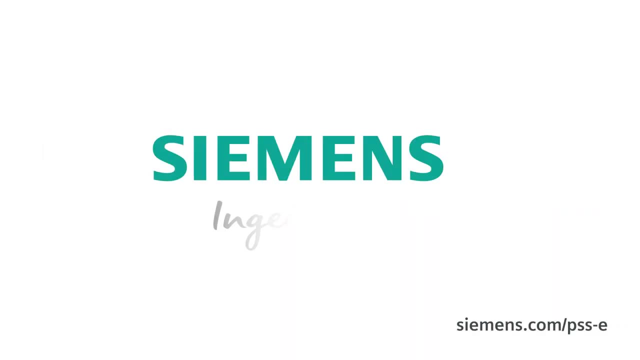 the stability of the system. These are just a few of the many features of Siemens PTI's comprehensive high-end analysis software. PSSE can help your transmission system planning to give you trusted benchmark results. Siemens Ingenuity for life.